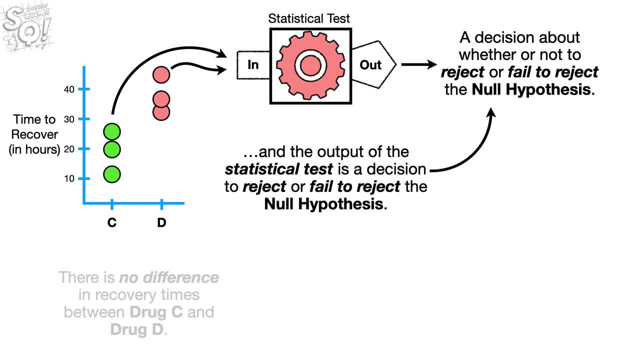 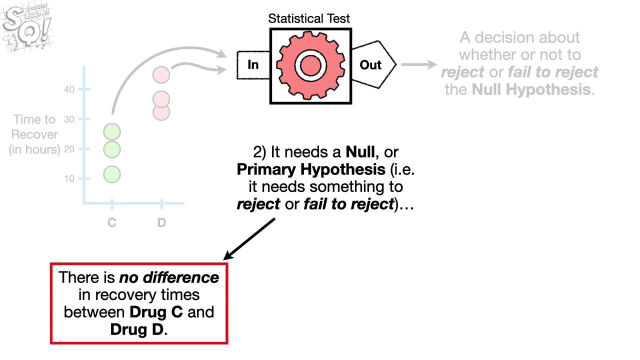 And the output of the statistical test is a decision to reject or fail to reject the null hypothesis. A statistical test needs three things. One, it needs data. Two, it needs a null or primary hypothesis, ie it needs something to reject or fail to reject. 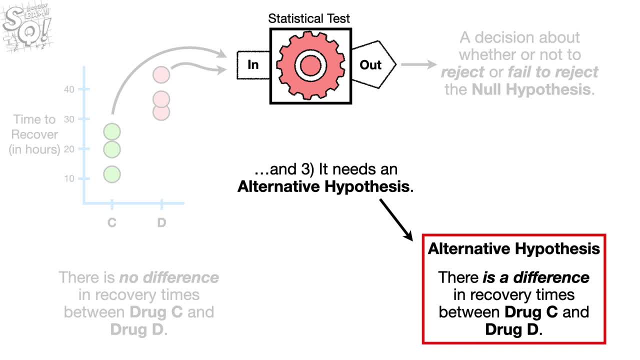 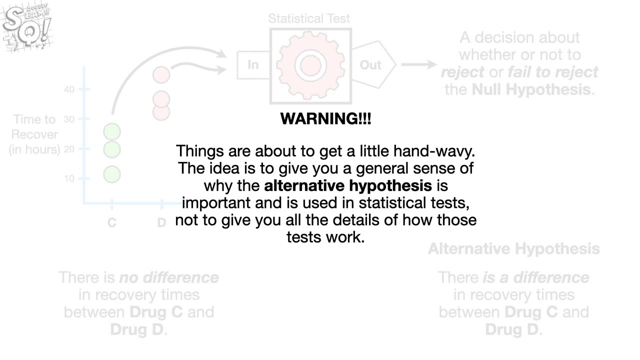 And three, it needs an alternative hypothesis. In this case, the alternative hypothesis is simply the opposite of the null hypothesis. Warning Things are about to get a little hand-wavy. The idea is to give you a general sense of why the alternative hypothesis is important. 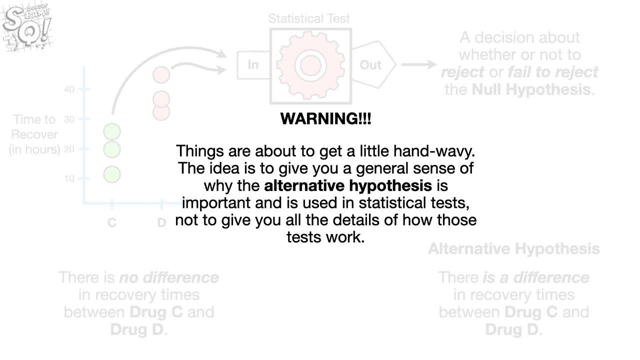 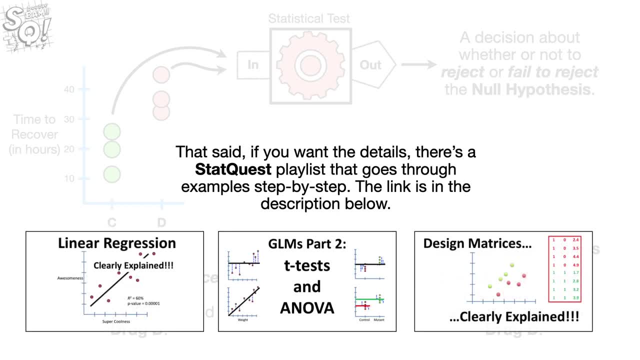 and is used in statistical tests, not to give you all the details of how those tests work. That said, if you want the details, there's a StatQuest playlist that goes through examples step by step. The link is in the description below. 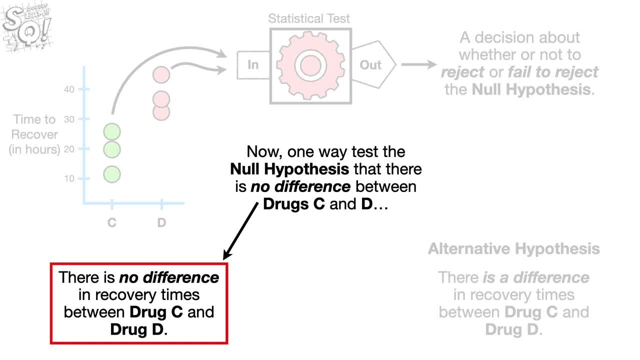 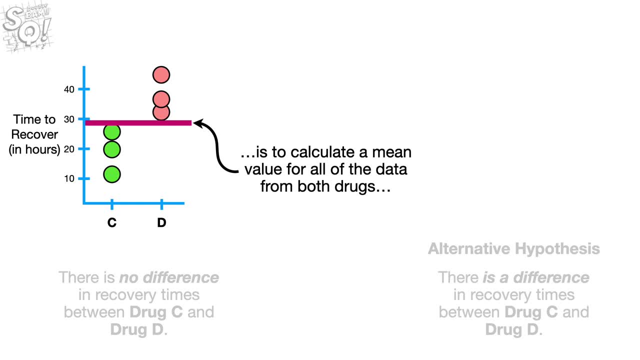 Now one way to test the null hypothesis that there is no null hypothesis is to use the null hypothesis- The null hypothesis that there is no difference between drug C and D- is to calculate a mean value for all the data from both drugs and calculate the distances between each observation and the mean. 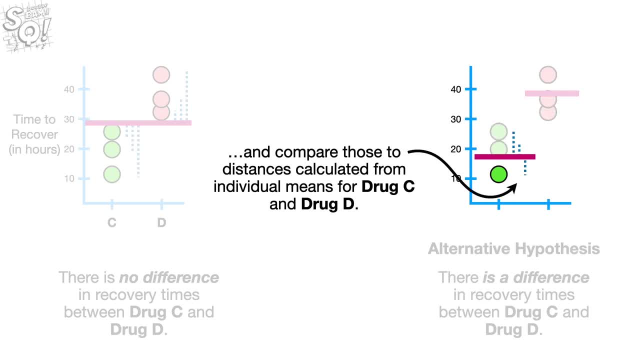 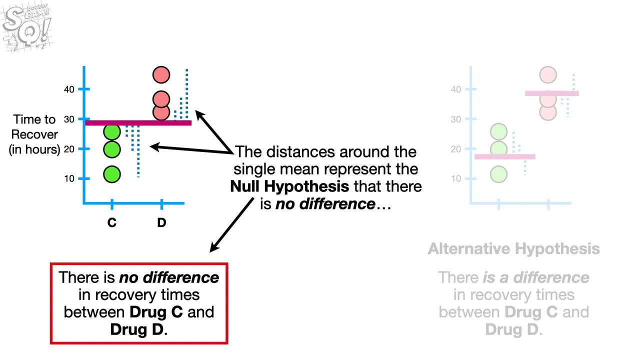 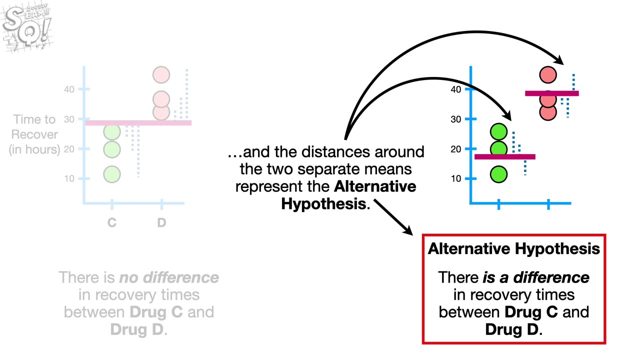 and compare those to distances calculated from individual means for drug C and drug D. The distances around the single mean represent the null hypothesis that there is no difference, And the distances around the single mean represent the null hypothesis that there is no difference. distances around the two separate means represent the alternative hypothesis. If the distances 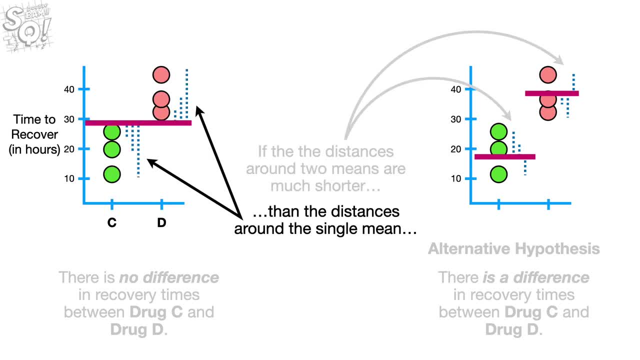 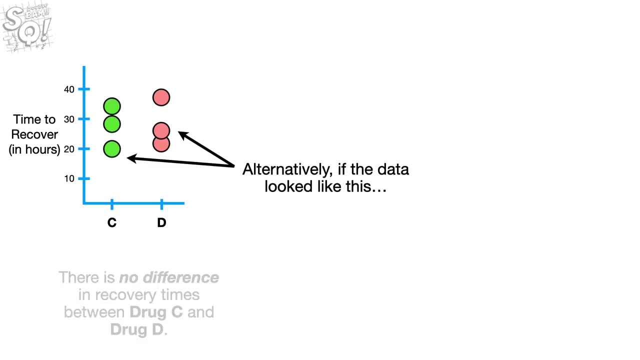 around two means are much shorter than the distances around the single mean, then that suggests that using two means to summarize the data makes more sense than using one. So we reject the null hypothesis. Alternatively, if the data looked like this and the distances 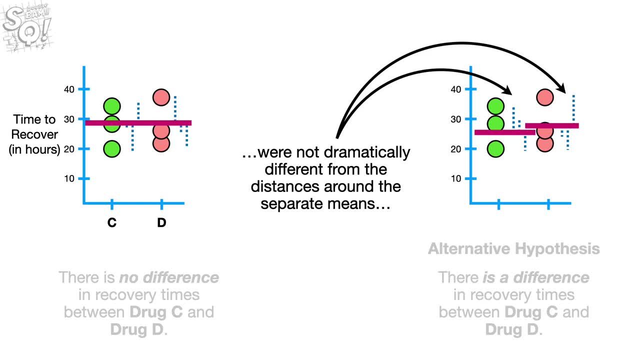 from the single mean were not dramatically different from the distances around the separate means, then that would suggest that the difference between two means only reflects little random things that we can't account for. For example, it could be that the subtle difference in the means is due to this one guy getting less exercise than everyone else If he had exercised just a. 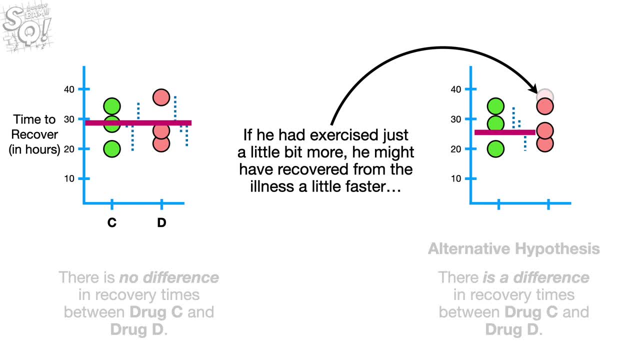 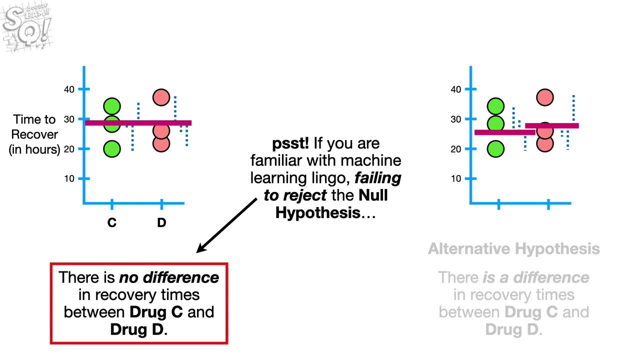 little bit more, he might have recovered from the illness a little faster, And then we would no longer see a difference between the two means. So in this case, we would fail to reject the null hypothesis- Psst, If you're familiar with machine learning lingo- failing to reject the null hypothesis. 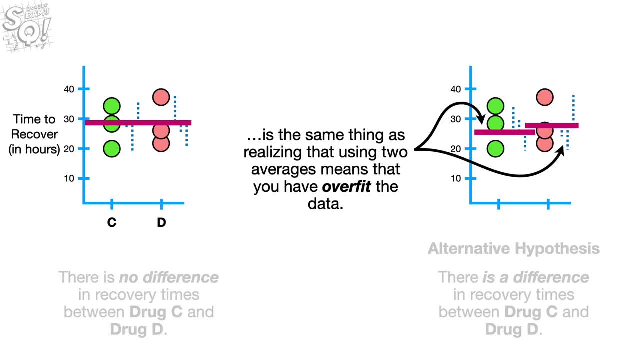 is the same thing as realizing that using two averages means that you have overfit the data. If you're not familiar with machine learning lingo, ignore what I just said Or, better yet, check out the machine learning stack quests. Note: when we only have two groups of data, the alternative hypothesis is pretty obvious. 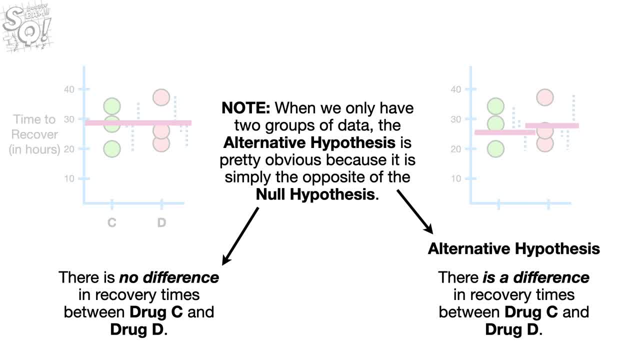 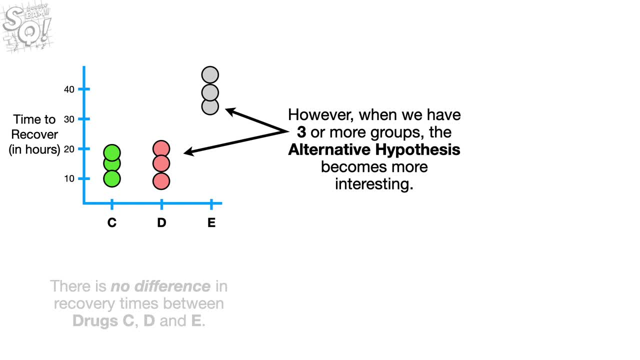 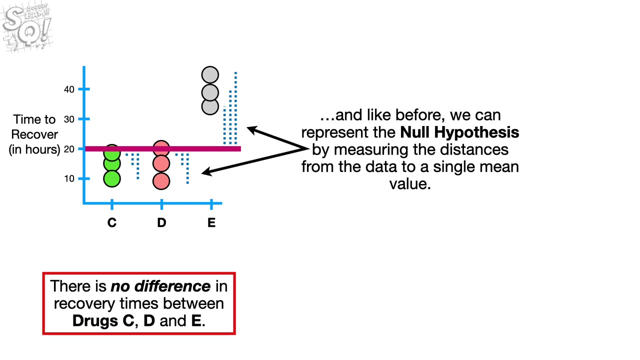 because it is simply the opposite of the null hypothesis. However, when we have three or more groups, the alternative hypothesis becomes more interesting. In this case, the null hypothesis is that there is no difference between drug C, D and E And, like before, we can represent the null hypothesis by measuring the distances from. 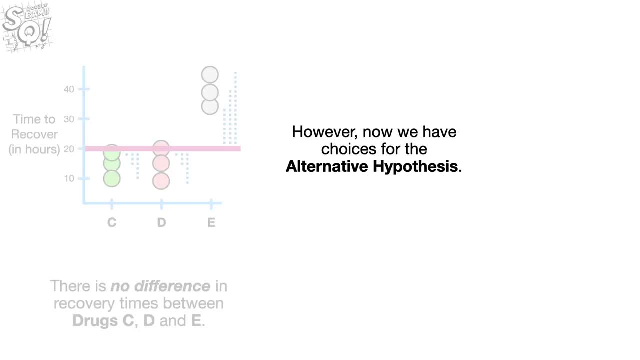 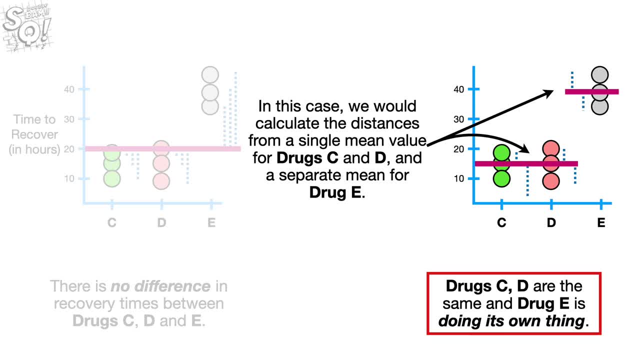 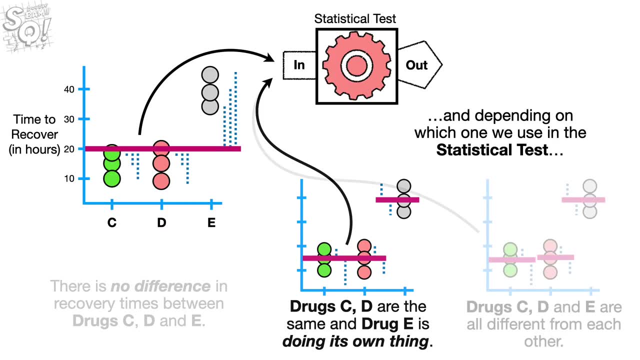 Or the alternative hypothesis could be that there is no difference between drug C, D and E, Or the alternative hypothesis could be that there is no difference between drug C, D and E E. So far, we have two different alternative hypotheses, And depending on which one we 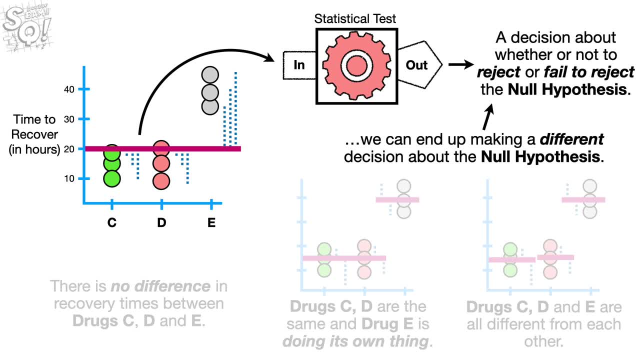 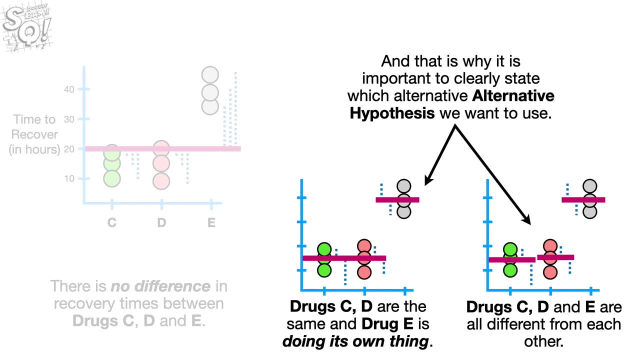 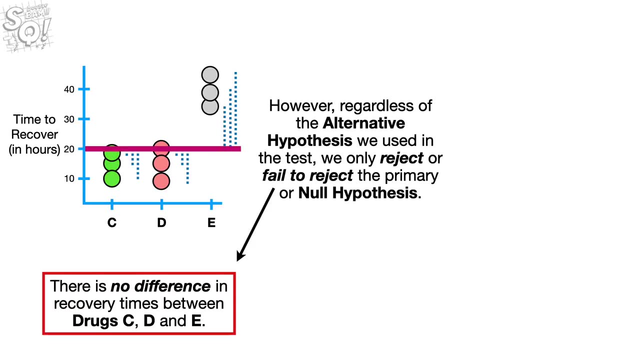 use in the statistical test, we can end up making a different decision about the null hypothesis, And that is why it is important to clearly state which alternative hypothesis we want to use. However, regardless of the alternative hypothesis we used in the test, we only reject or fail to reject the primary or null hypothesis. If we tested the null, 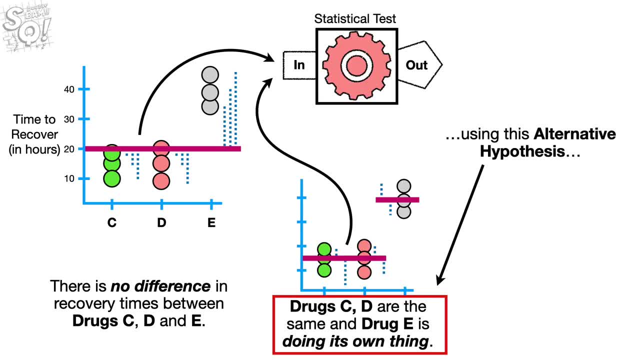 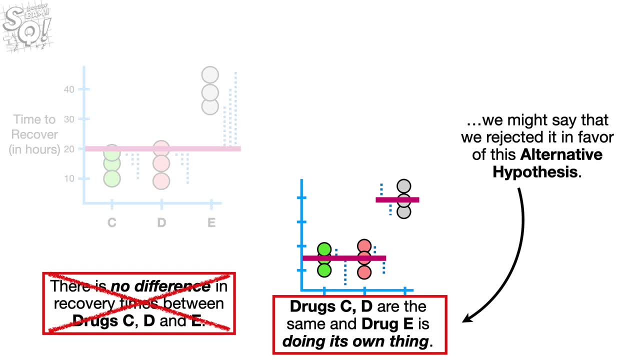 hypothesis, using this alternative hypothesis and we rejected the null hypothesis. we might say that we rejected it in favor of this alternative hypothesis. However, we would still not say we accept the alternative hypothesis because, just like we saw in the stack question, we reject the null hypothesis. 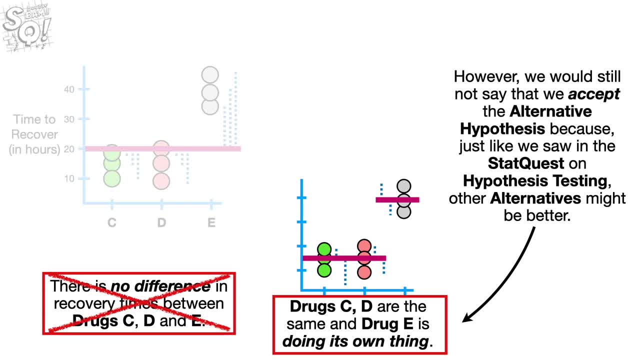 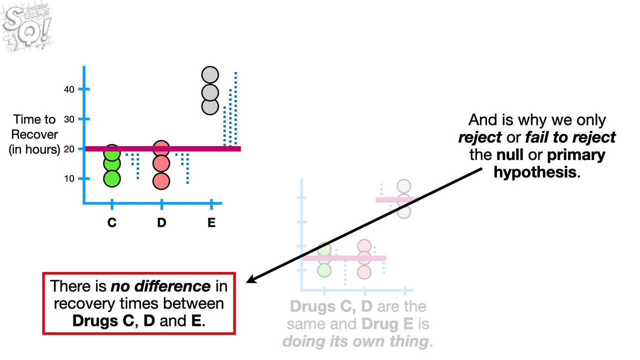 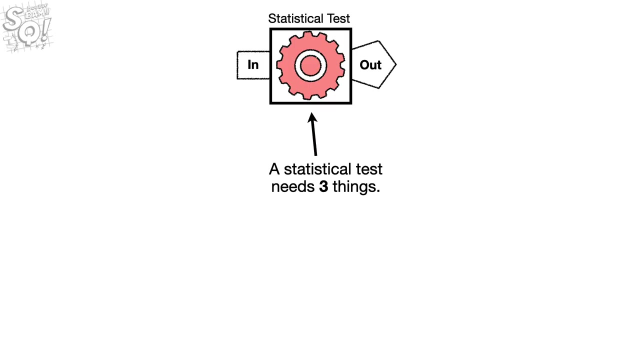 In other words, there are too many possibilities to test to know if we have accepted the correct one, And this is why we only reject or fail to reject the null or primary hypothesis BAM. In summary, a statistical test needs three things: 1. It needs data. 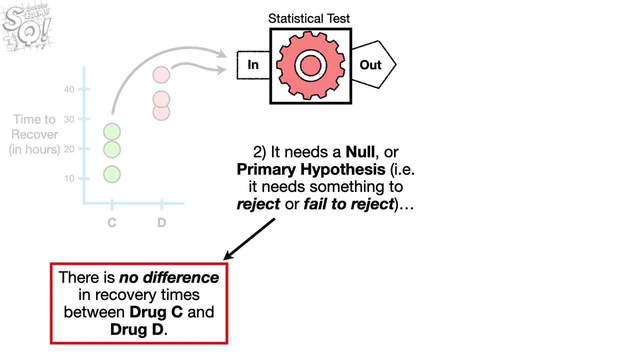 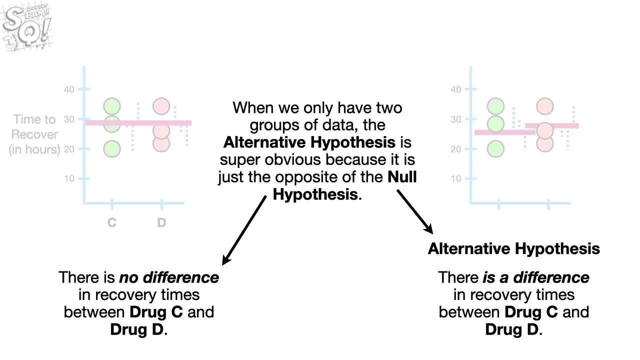 2. It needs a null or primary hypothesis. And 3. It needs an alternative hypothesis. When we only have two groups of data, the alternative hypothesis is super obvious because it is just the opposite of the null hypothesis. But when we have three or more groups, we 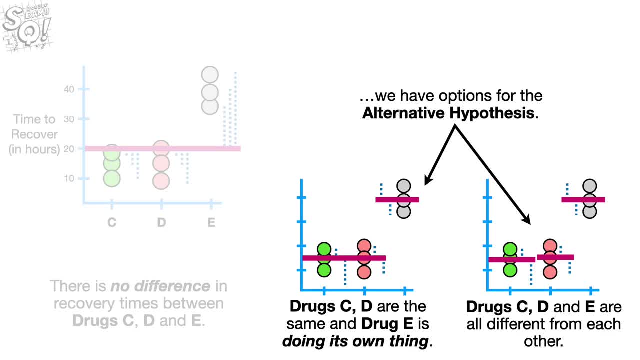 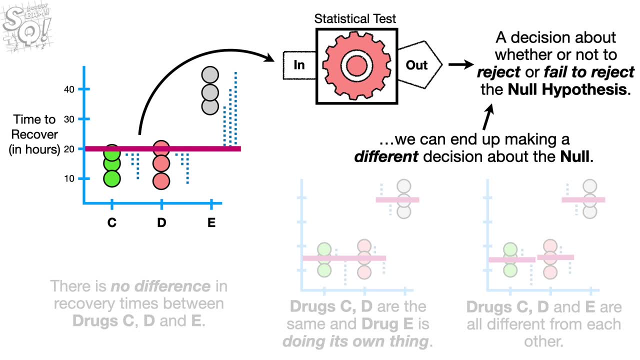 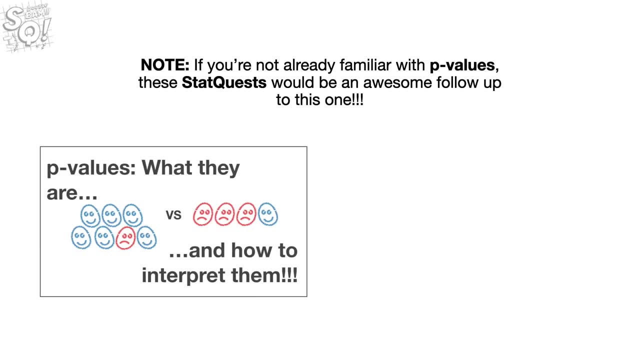 have options for the alternative hypothesis And, depending on which one we use in the statistical test, we can end up making a different decision about the null Double BAM. If you are not already familiar with p-values, these stack quests would be an awesome follow up to this one. 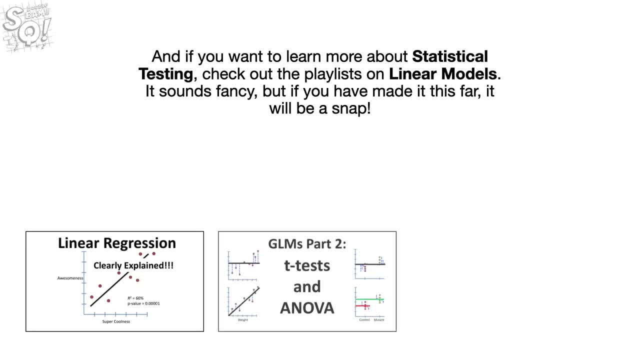 And if you want to learn more about statistical testing, check out the playlist on linear models. It sounds fancy, but if you've made it this far, it will be a snap. Now it's time for some simple data testing. The linear cows are really fast.